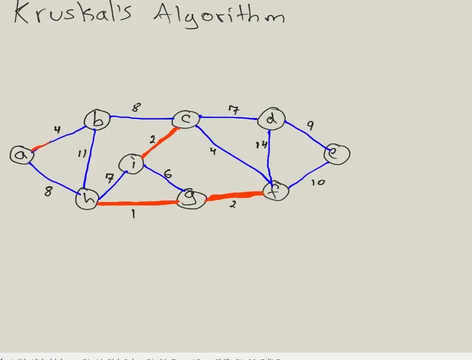 So let's go ahead and pick A and B, Like so, and let's also pick C and F, because this will not form a cycle in our in our tree. Okay, All right. so next number up is 5.. Do we have 5 anywhere? 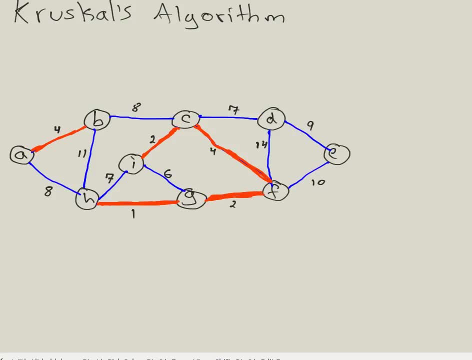 No, we do not. Then we have 6.. We have one 6, but, as we said, we can't pick an edge- UV that will form a cycle. It's because this two edges belong in the same tree. See, I and G are part of the same tree. so we cannot pick this edge, because if we do like so, 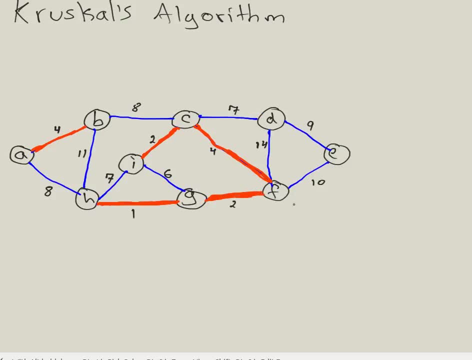 then we'll have a cycle, which is not allowed. Okay, next number up is 7.. We have two 7s, Um. this 7 will form a cycle, so we can't pick that. So the only other choice we have left is the edge C, D. 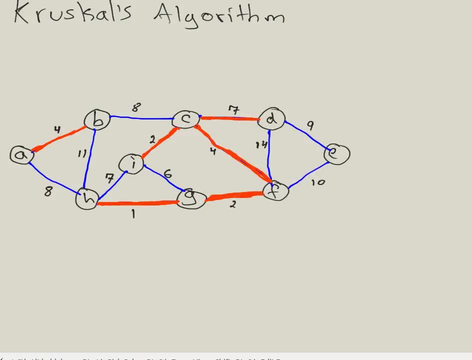 So let's go ahead and pick this. So now the edge C D, The edge C D are in our tree. Okay, Next number up is 8.. We have two 8s. Um, it doesn't matter which one you pick. 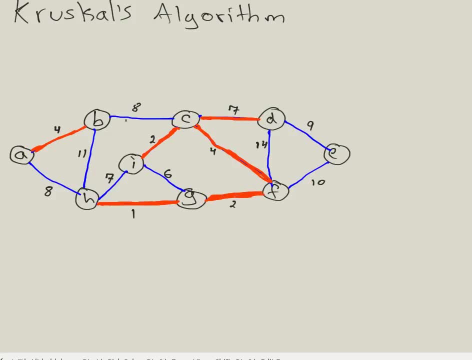 Um, none of them will form a cycle as far as I can see. Nope, doesn't look like it, So let's go ahead and pick this edge right here. B and C, Okay, And, as you can see, you can have more than one minimum spanning trees. 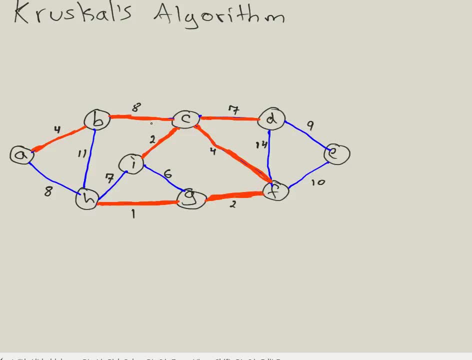 If we Have picked this eight, then we wouldn't be allowed to pick um this eight, which would be a different tree than if we have, because if we chose this one it would be a different tree spanning tree than if we have chosen this one. 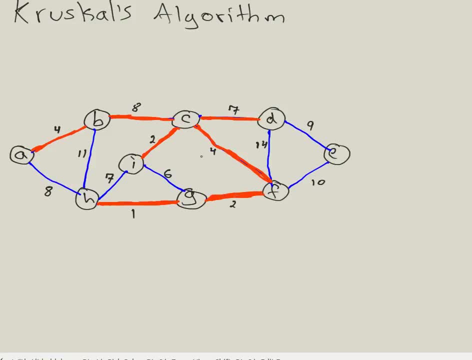 So moving on, we have: uh. next number up is nine. We have one one nine, So we have to pick that one because you will not form a cycle in our graph. So the edge D and E are next to be picked. 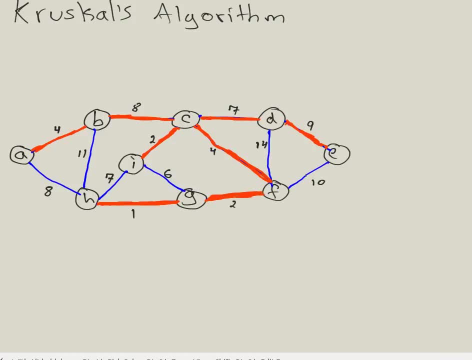 And the next number up is 10.. It's right here, but this will form a cycle, So we skip over that. Then we have 11.. This will also form a cycle which we can have, So we don't pick this. and 12,, no 13,, no 14..